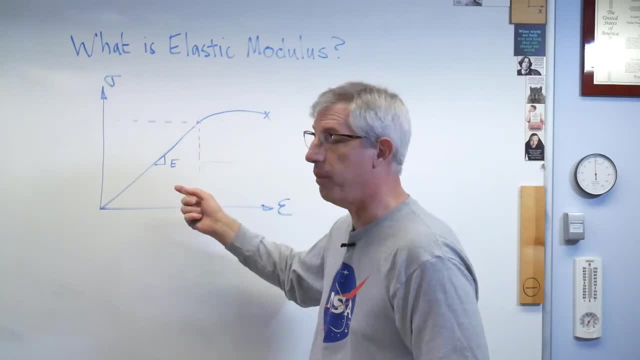 And I pull, but I only pull up to about there and I let go. it'll return to its original length. And I pull, but I only pull up to about there and I let go. it'll return to its original shape. That's what elastic means. 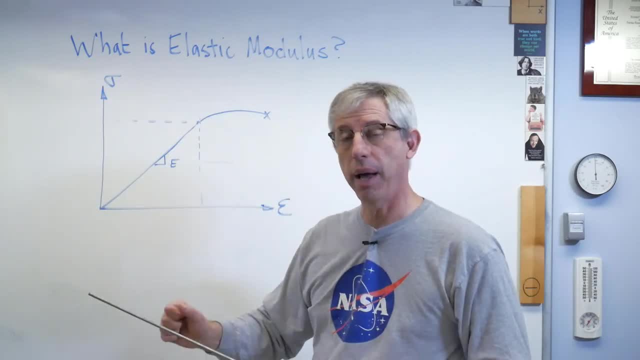 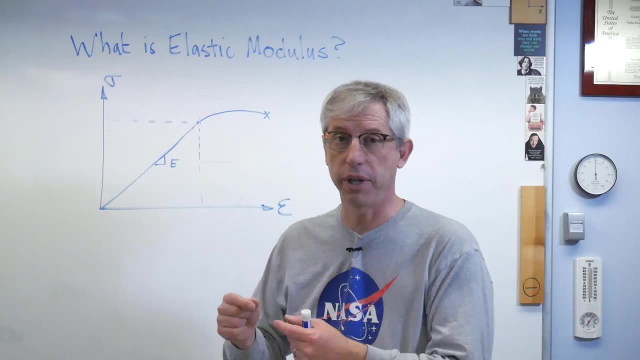 If I go out here, pull hard enough, I'm going to permanently deform it and that's called plastic deformation. So if you let go of the material, your test sample, and it goes back to its original shape, that was elastic deformation. 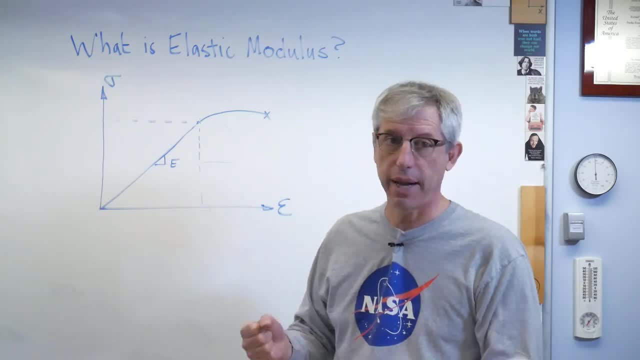 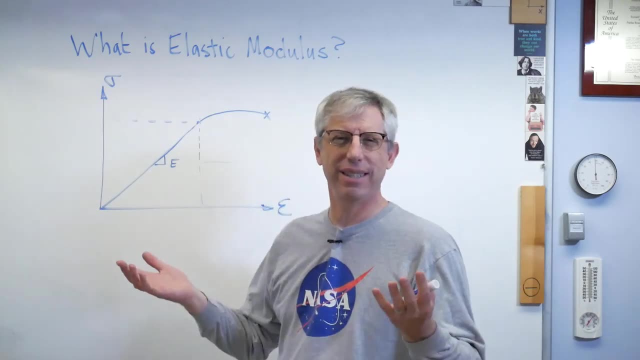 If you pull it so hard that it's permanently deformed, that's plastic deformation. So that slope of that curve is elastic, modulus. Ehhh, okay, I mean that's correct with a, without necessarily being helpful. Okay, let's try something else here. 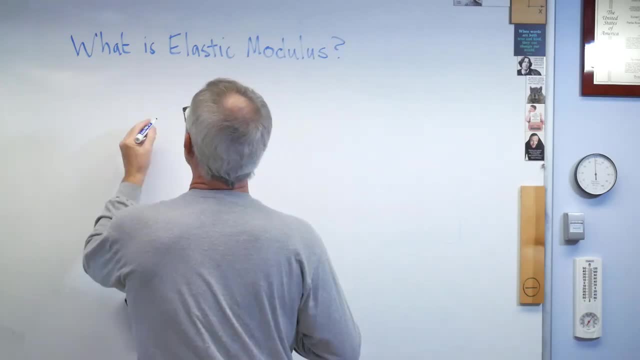 Imagine you have a beam And maybe, let's see, it's like an I-beam. Okay, See if I can do this real quick. Well, look at that, he got it. Huh, Look at that, there's an I-beam for you. 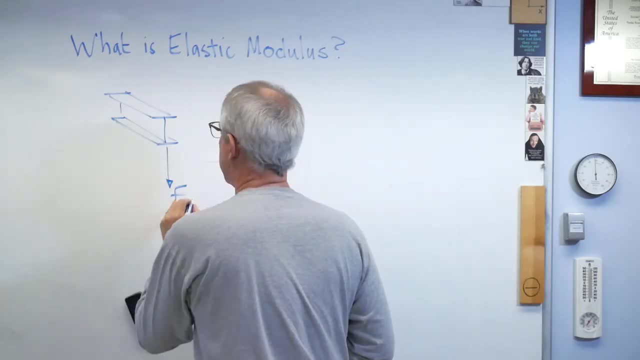 And you put a big load on the end of it. And you put a big load on the end of it. Alright, there's a construction site right there, just almost on the other side of my window. Alright, there's a construction site right there, just almost on the other side of my window. 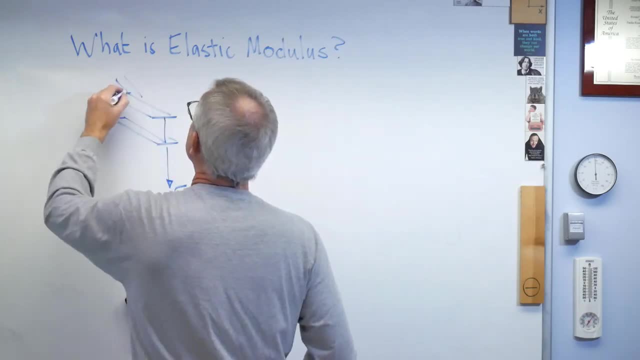 Alright, there's a construction site right there, just almost on the other side of my window. Yeah, there are beams and stuff all over the place here And it's connected to something over here. This is: this is a clamped boundary condition, I guess. 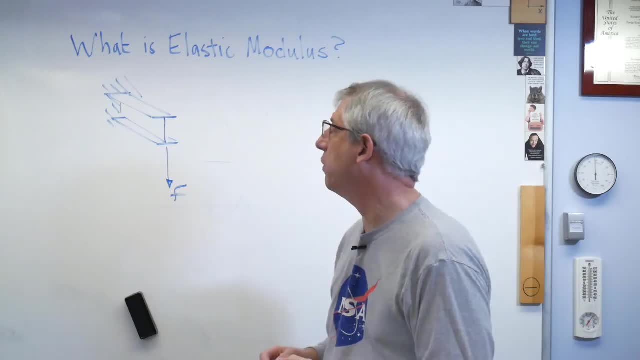 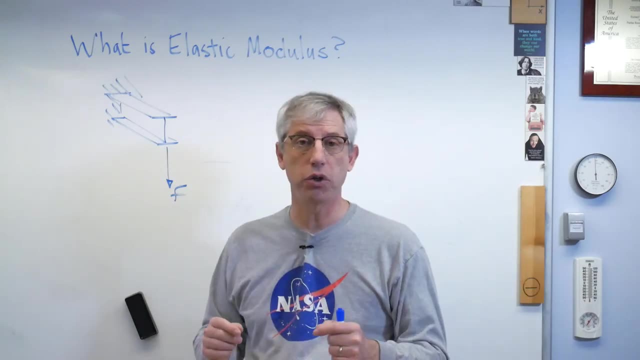 This beam. it's stiff but it's not rigid. Okay, if you put a big enough load on it it'll move noticeably Well. the beam bends. it's got stiffness that comes from two different sources: One is the shape of the beam and one is the material. 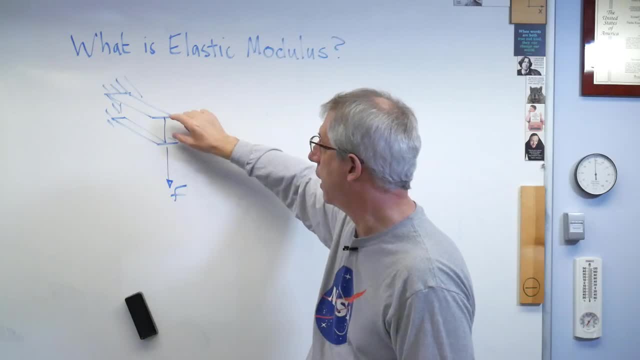 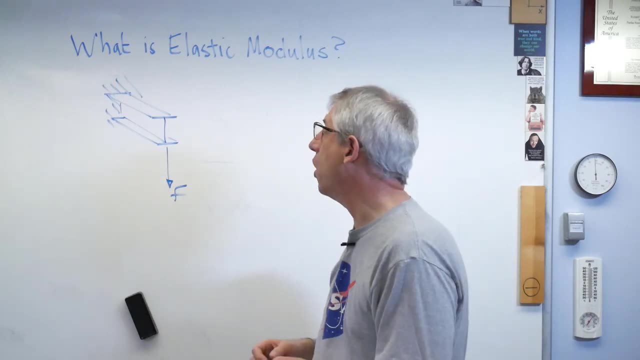 So the reason I-beams are made like they are is because when you move something, it moves back right. Right, that's true. because when you move material out towards the top and the bottom of them, they get stiffer, they get more able to resist load, they get stiffer and 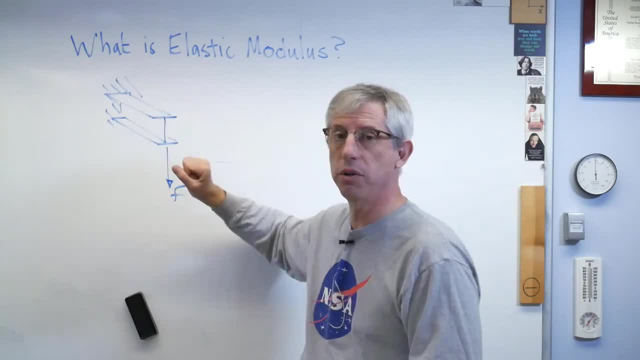 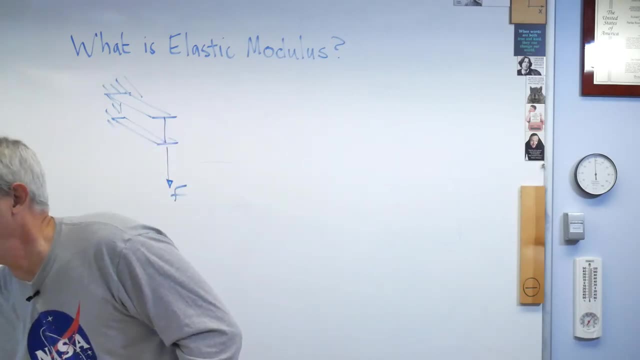 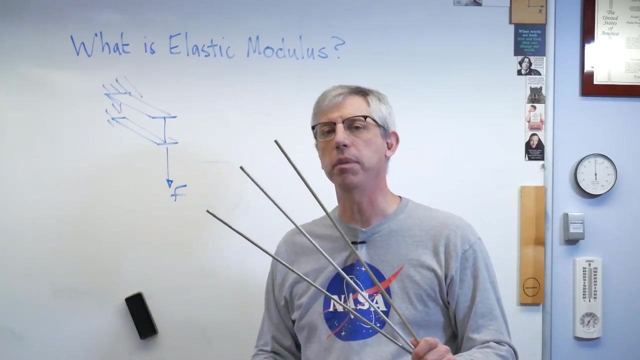 stronger, so that's stiffness due to shape. but you can also change the material. so here's the. I've got three rods. here they're because I live in the United States. they're three feet long and they're a quarter inch in diameter. they're about a meter long and six point three, five millimeters in diameter. if 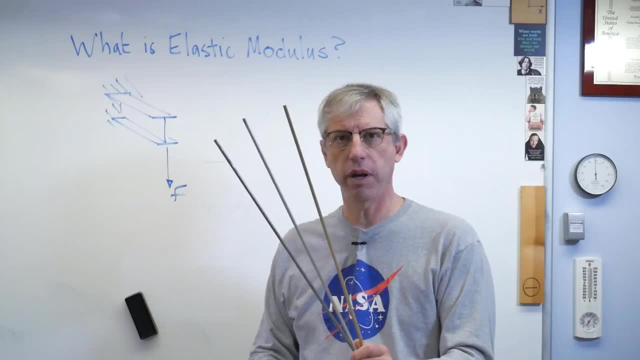 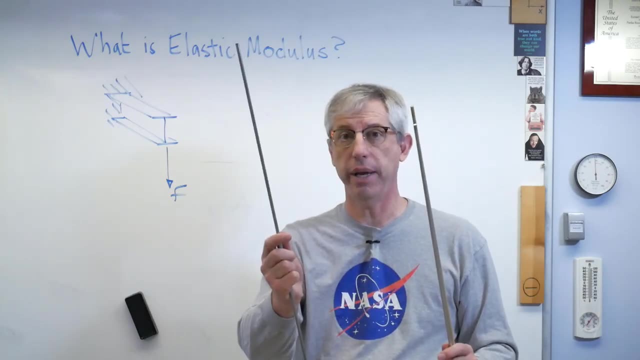 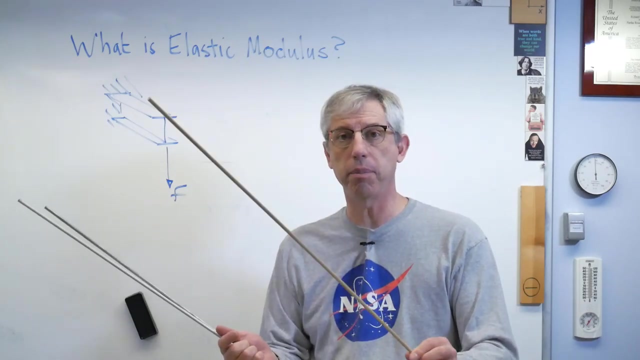 you want to use not silly English units. there's three of them in there, right? the shapes are absolutely identical- as identical as I could get them right. this one is made out of steel, this one's made out of aluminum and this one is made out of a wood called poplar. all right, it's a kind of hard wood. it's harder than than. 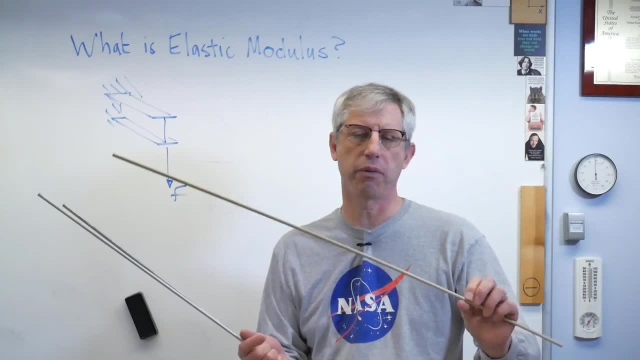 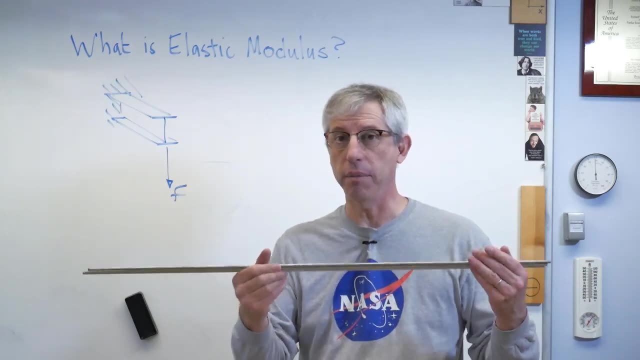 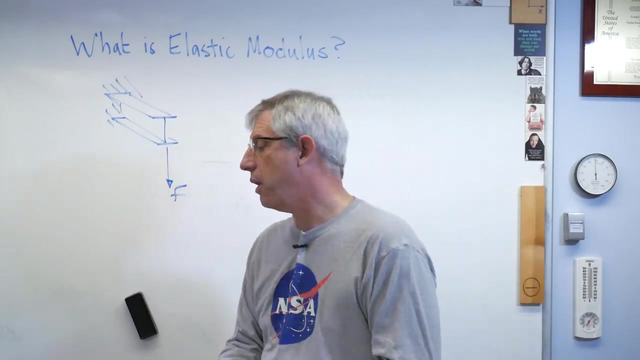 pine, but not as hard as maple, gets used for a lot of furniture and cabinetry and things. it's nice stuff. so, apart from their material, they are absolutely identical- as identical as I could get them. they're circular rods, same length, same diameter. so just I'll. 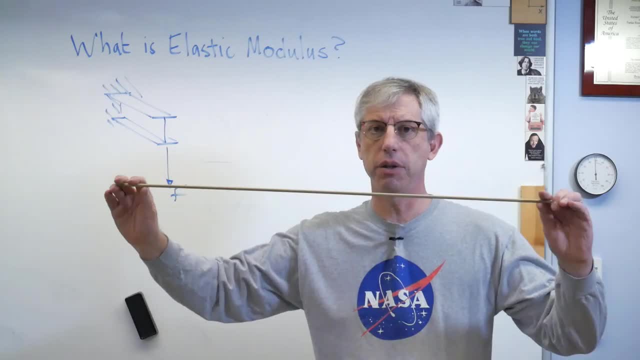 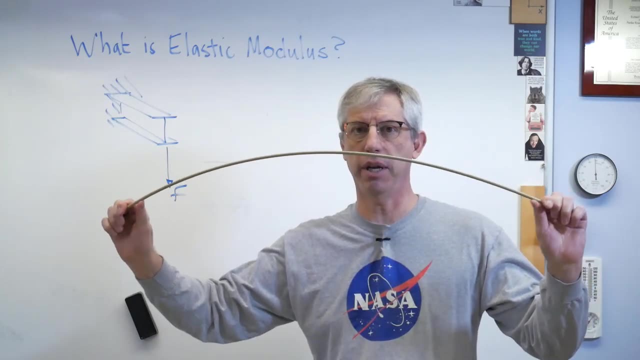 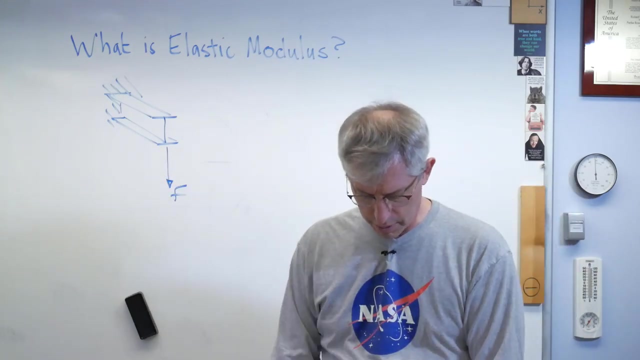 just do it this way. okay, here's the wooden rod. this is poplar wood and it's super easy to bend. okay, just with my fingertips, I can bend it very, very easily. okay, this is not very rigid. it's very flexible. all right, let's check. if it doesn't resist, well, I'm gonna bend it. okay, now here's the Rather Slow. 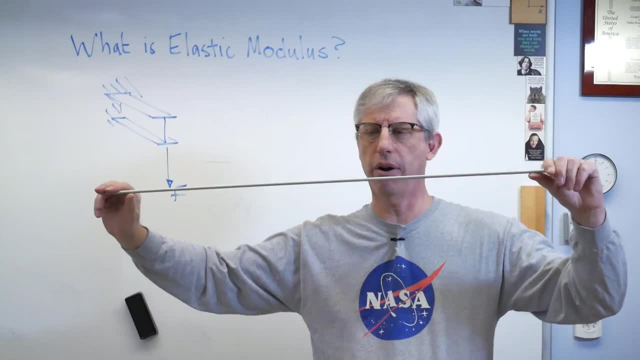 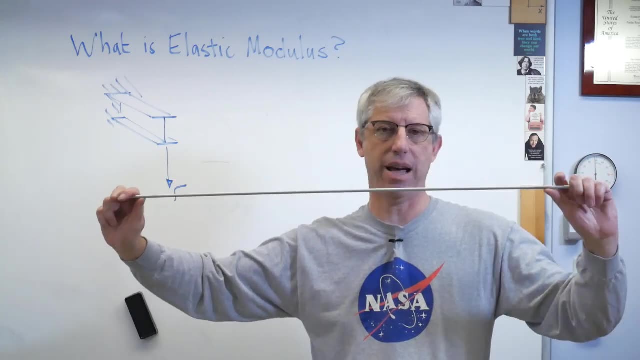 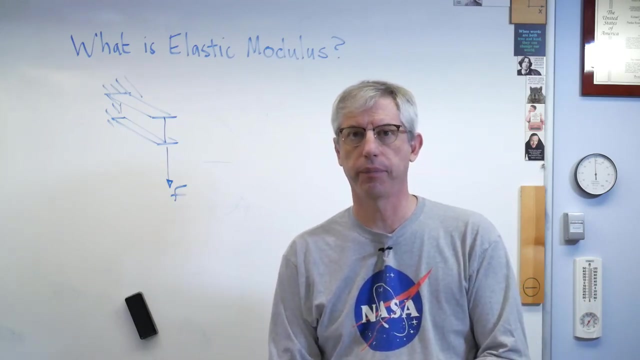 change. now here's the aluminum rod. this one's a lot harder to bend. I'm having to push with my fingertips and I'm going to really dig in to get that bend there. they get that curvature there, okay. so let's go to the aluminum rod. sorry, this let's. 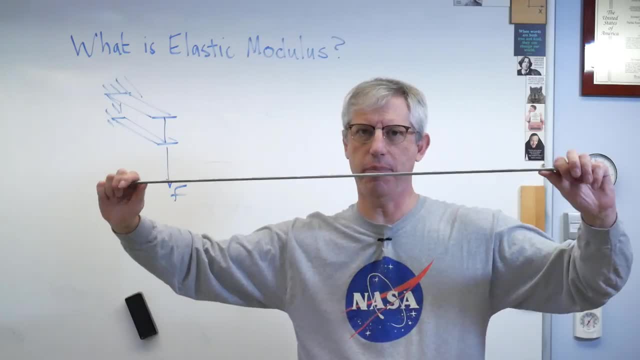 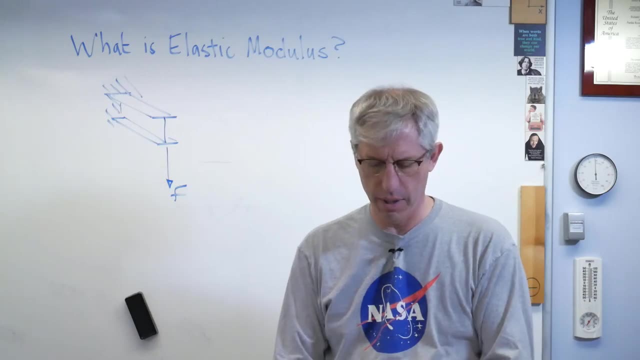 go to the steel rod. this one I can hardly bend at all. that's hurting, hurting my fingers, I can't see it. I repeat, so I'm going to put this on a wood, can't? I can't do that. so there's, that's all I can do. go back to the poplar. no, 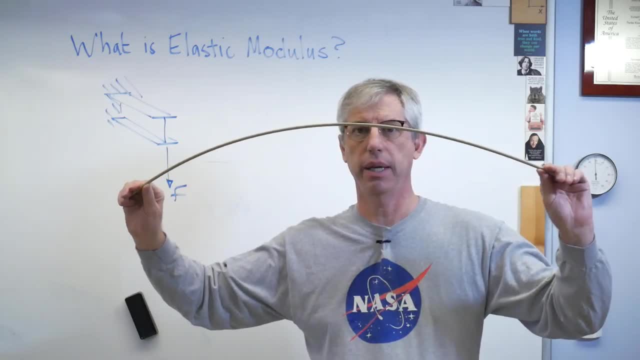 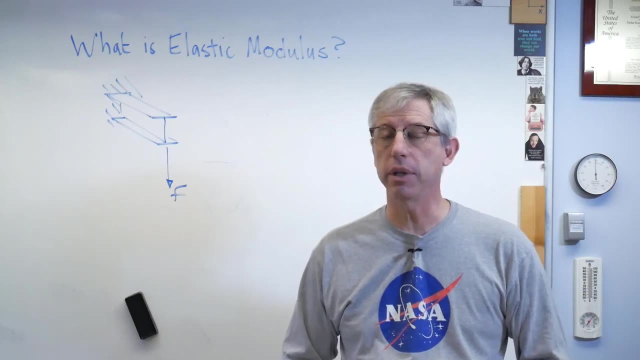 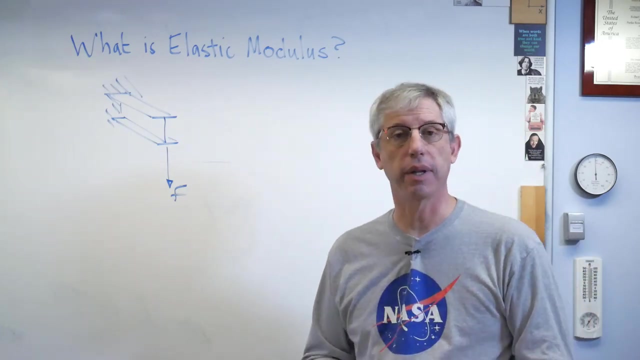 problem, very flexible. and because they are all the same size, they are all the same shape. the only difference between the three of them is the stiffness of the material. so everything in the engineering world gets a number, and elastic modulus is no different. it's defined by the letter E, right, and we E. 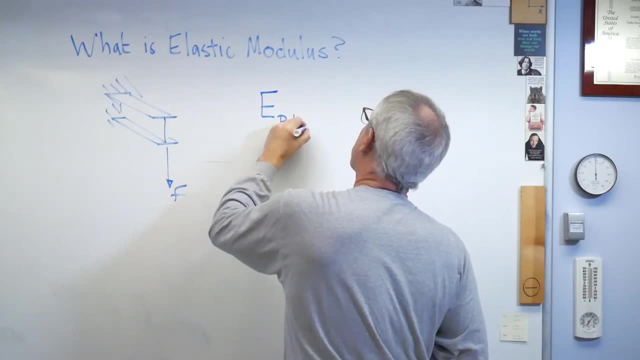 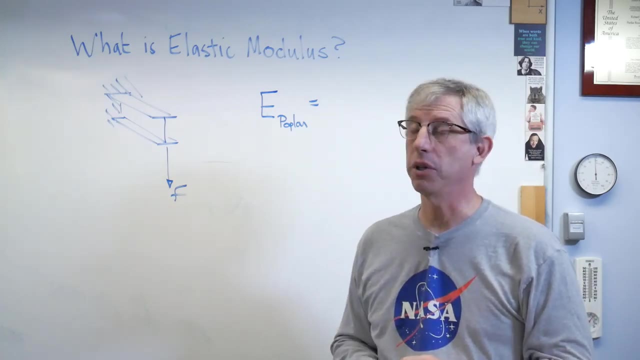 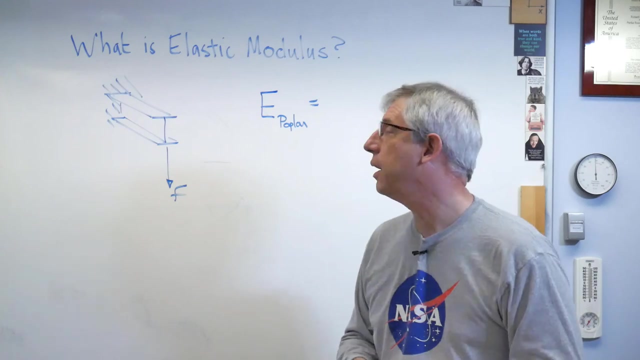 is for elastic. I guess here's elastic modulus for poplar. I'll write down that here in a second. one thing to note is in some old engineering books and some physics books you'll see this as a Y and the reason is it was originally called Young's modulus after some scientist or engineer named young, all modern. 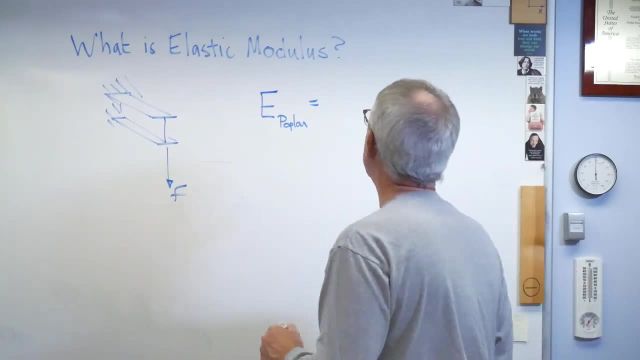 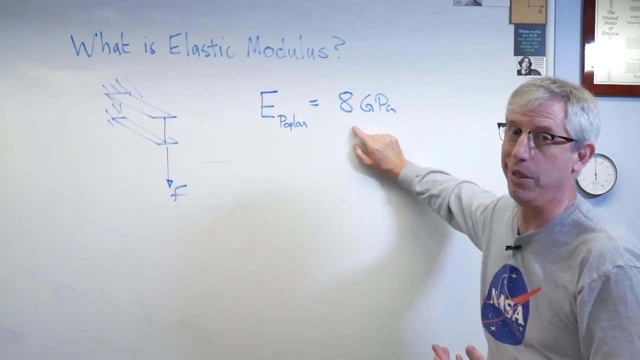 references call that an E and that's probably more makes more sense. so the elastic modulus of poplar is different from the elastic modulus of the poplar in metric units. it is about eight giga pascals now. I say about, because all trees are different, though the one on Matweb list. that is eight giga. 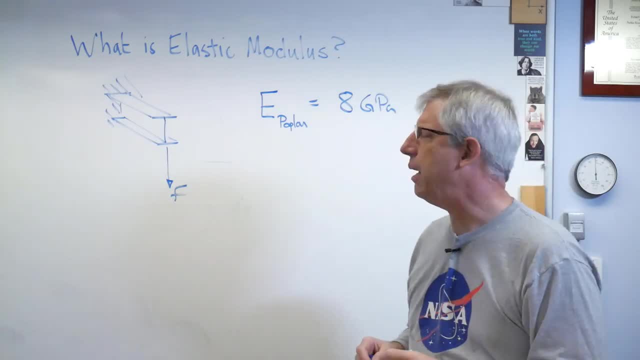 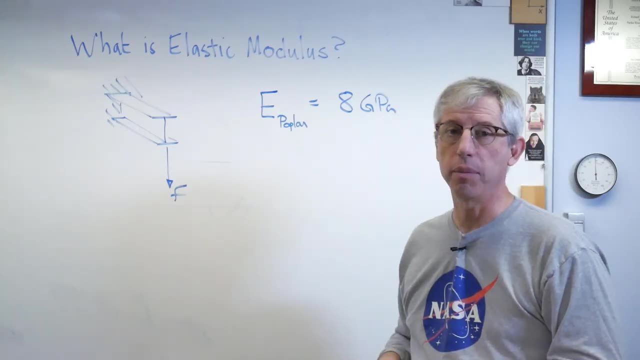 pascals, that's a big number. it's 8 billion pascals and all sorts Paschals. why is in units of pressure? well, it it's a units of force over area, because that's the units of stress, and then we're on the stress strain curve. so this: 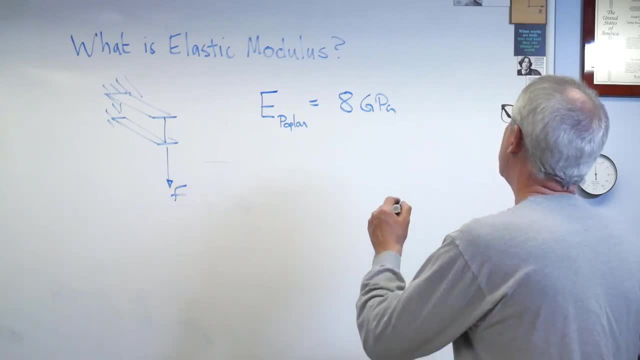 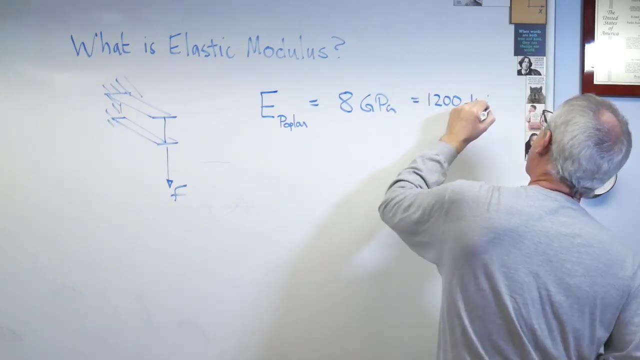 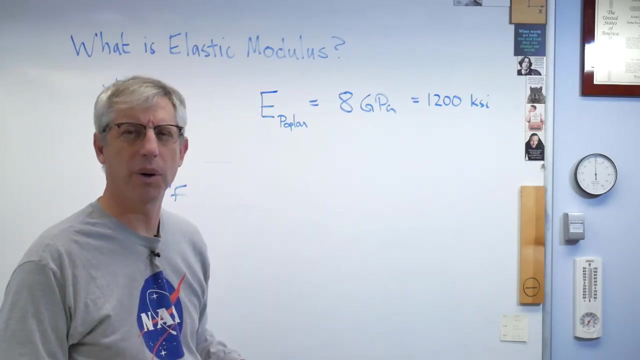 isn't really pressure, but it does have units that look like pressure. in English units it's about million PSI and you usually see this written as KSI, right? so it's again pounds: 1.2 million pounds per square inch. so 8 million big number, but it only. 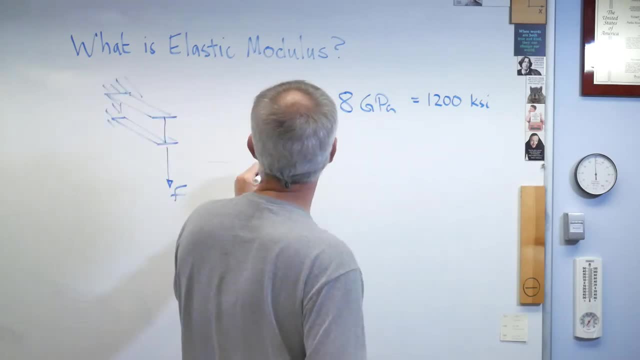 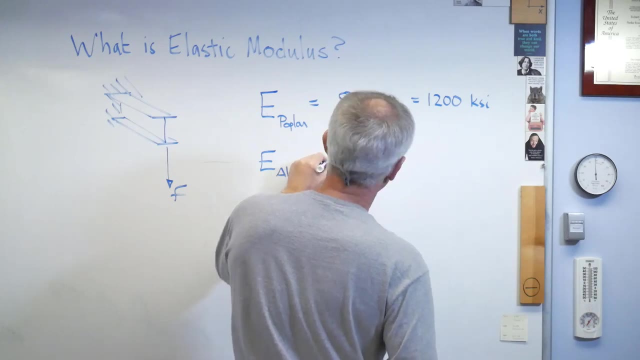 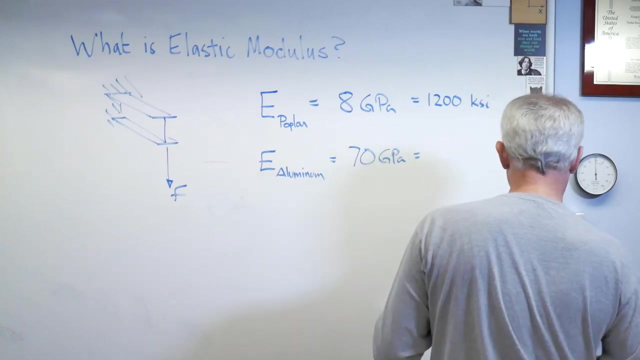 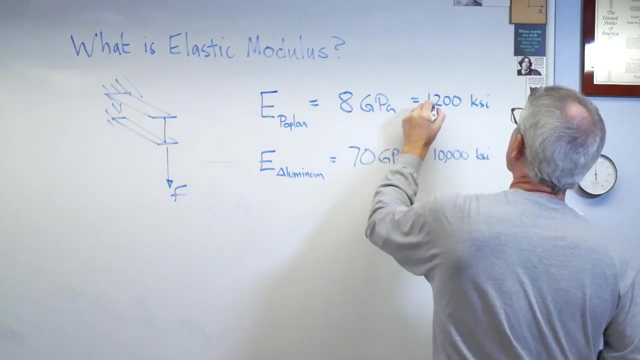 makes it only matters in comparison to the other materials. so let's take E of the aluminum- or aluminium, depending on where you are right now listening to this- and this is 70 gigapascals- much bigger number- and in English units that's about 10 million PSI or 10,000 KSI there. so much, much bigger number, okay. 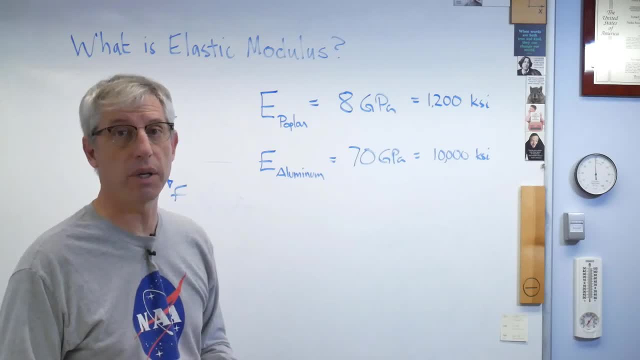 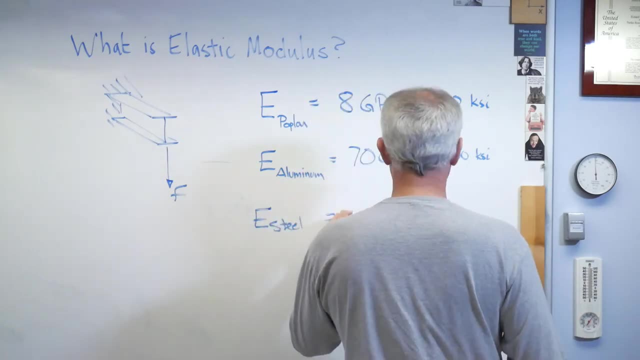 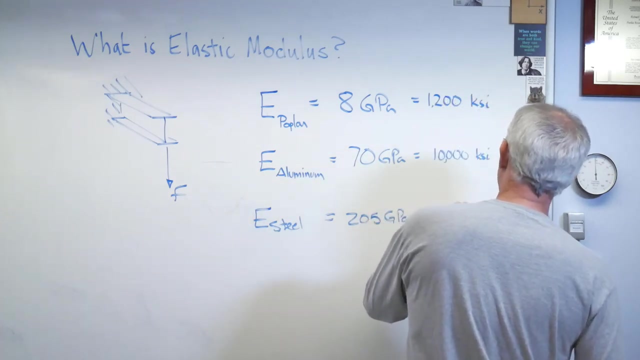 well, that explains it. that's why it's so much harder to bend that aluminum rod than it was to bend that wooden rod. and last one, let's go to steel, and that's two hundred and five gigapascals and that's about 30 million PSI. there's 30,000 KSI. so this explains. 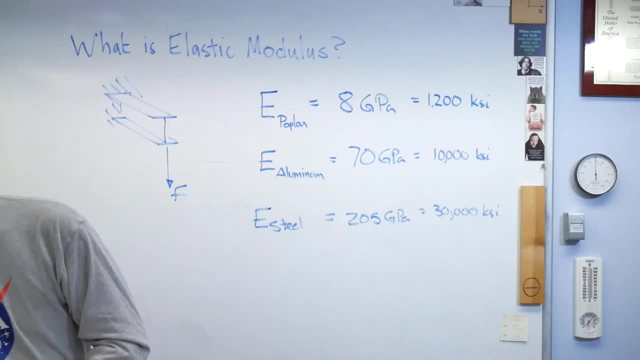 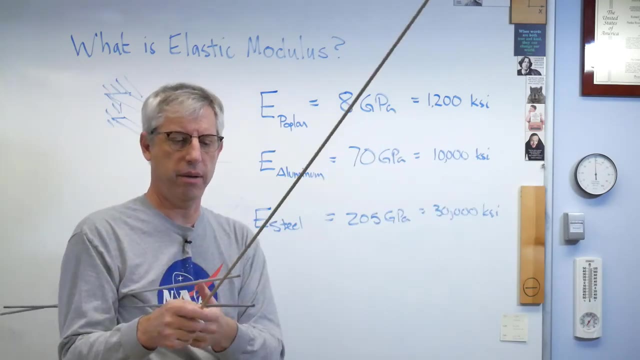 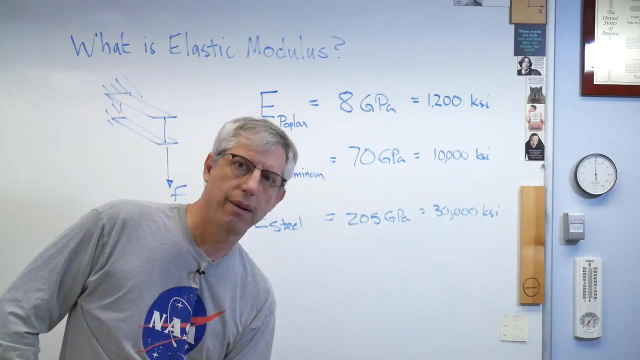 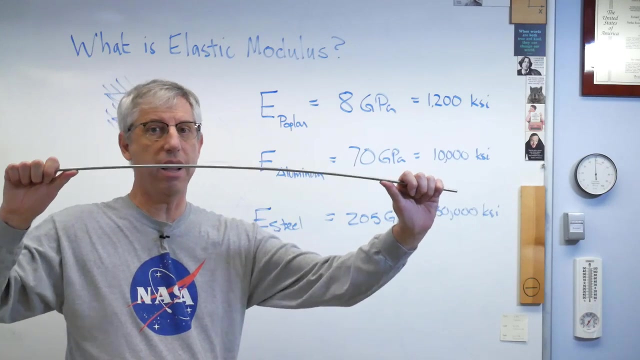 it. this, this right here, explains the difference in stiffness between these three rods. remember: aluminum, wood, real, real easy to bend. let's see if I can do this here again. aluminum, much easier to bend and steel pretty dang hard to bend. okay, with my hands there, I can just barely put a bend in, and it's.